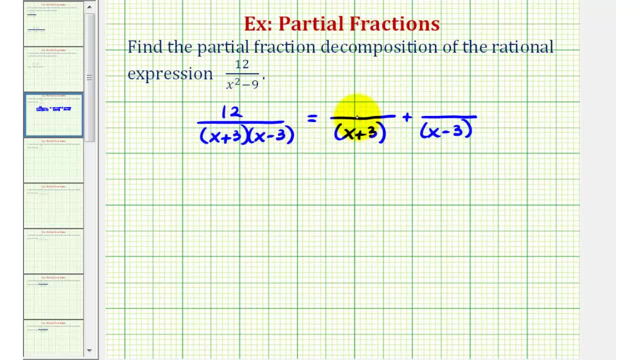 And again, because we have linear factors in our denominator. that means our numerators will be constants, which we don't know the values of right now. so we'll use the variable a for this numerator and b for this numerator, So we're using a single variable for the numerators. 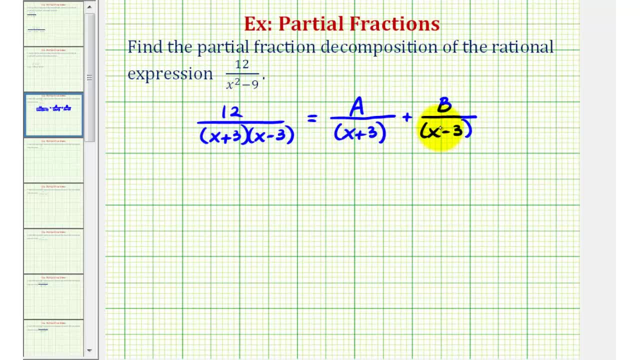 because we have linear factors in the denominator And now, if we can find the value of a and b, we'll have our partial fraction decomposition. So to solve this equation, we're going to clear the fractions by multiplying both sides of the equation by the least common denominator, which would be: 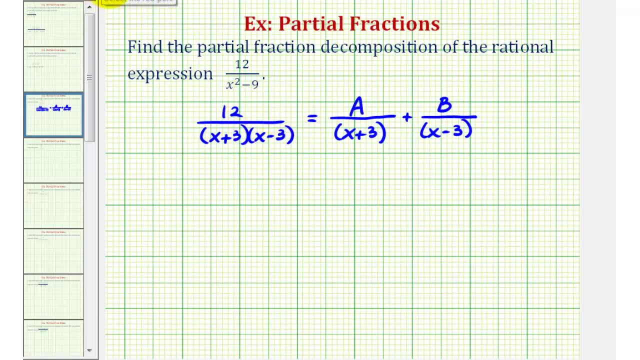 the quantity x plus three times the quantity x minus three. Notice on the left side: when we multiply x plus three over x plus three simplifies to one, and so does x minus three over x minus three. so we're left with 12 equals. 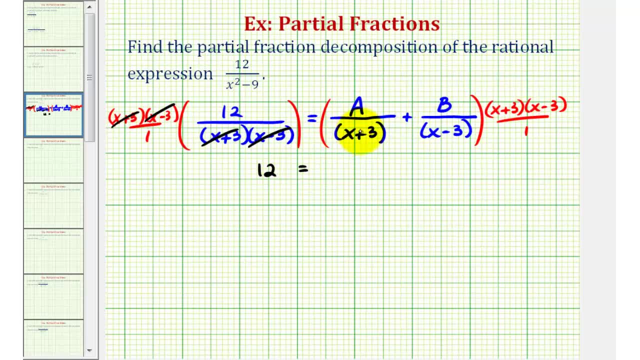 and on the right side. for this first product, x plus three over x plus three would simplify out, leaving us with a times the quantity x minus three. and then for the second product, notice how x minus three over x minus three simplifies to one. 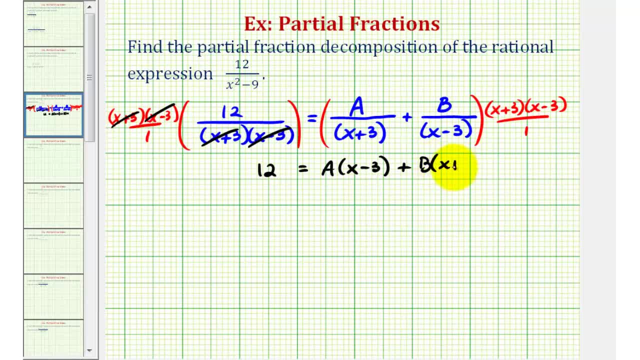 so we'd have b times the quantity x plus three. This equation here is called the basic equation which we want to solve, to find the value of a and the value of b. And there are a couple ways to solve this of a and b. 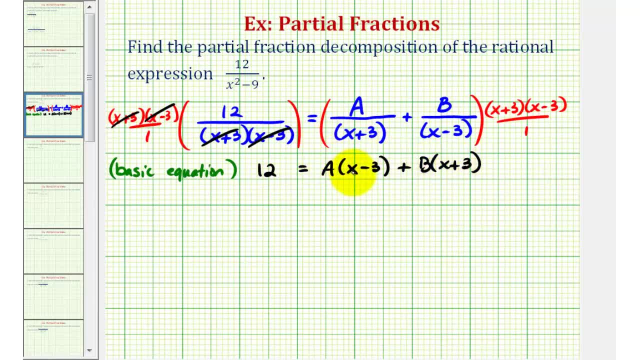 One way is to multiply out the right side, combine like terms and then set the coefficients of like terms on the left side of the equation and the right side of the equation equal to each other, to form a system of equations, or which we'll do in this example. 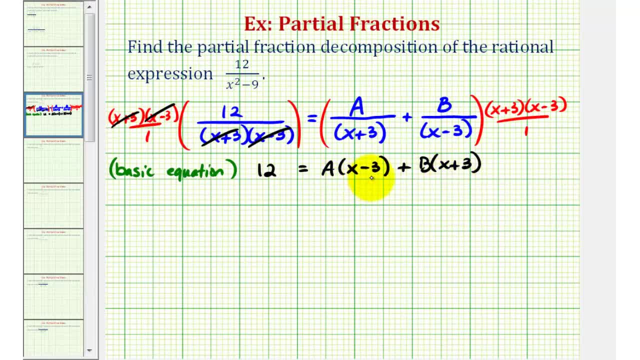 we can select convenient values of x and then perform substitution in order to find the values of a and b. When I say convenient values of x, we're going to pick values of x that make the factor x minus three, or the factor of x plus three, equal to zero. 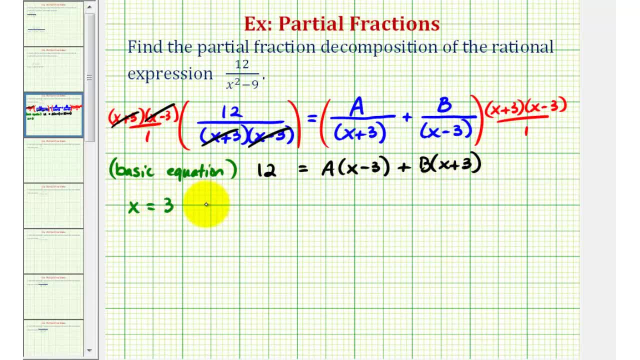 For example, if we select x equals three and perform substitution, that would give us the equation 12 equals. well, if x is equal to three, we would have a times zero, which is equal to zero. Well, this is eliminated.